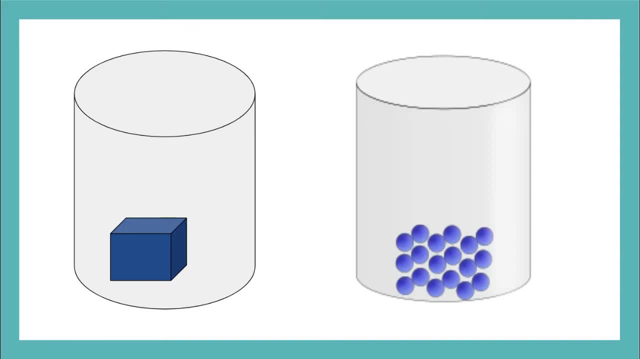 usually in a pattern, and they hardly move. They may vibrate or jiggle, but for the most part they are fixed in place. That is why it is so hard to compress or squish a solid. Liquids are able to flow and move. 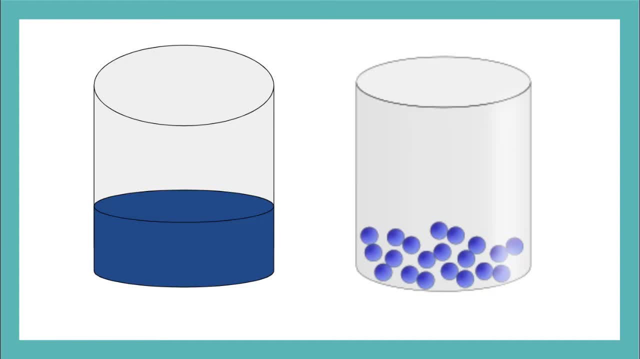 Gases can change their shape because the atoms and molecules are not fixed. They are able to slide past each other and they move faster than particles in a solid. The particles in a liquid have more free space between them than in a solid. This makes it easier for a liquid to flow and change shapes. 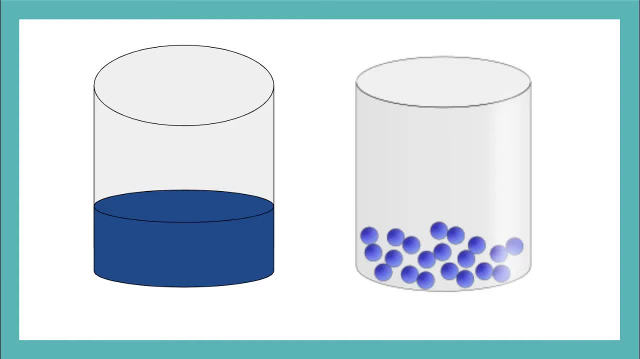 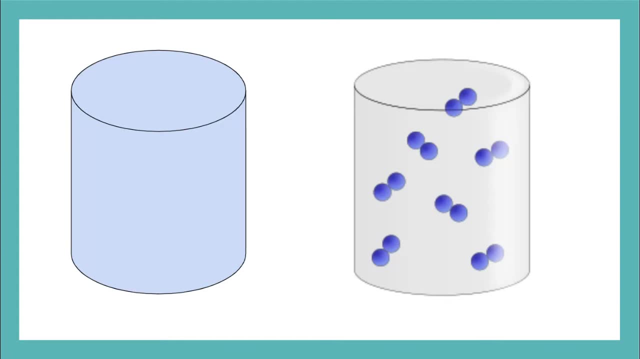 But since the particles are still close together, a liquid is hard to compress or make smaller. Gases are able to change their shape and their volume because the atoms and molecules can move freely. Gases are able to change their shape and their volume because the atoms and molecules can move freely. 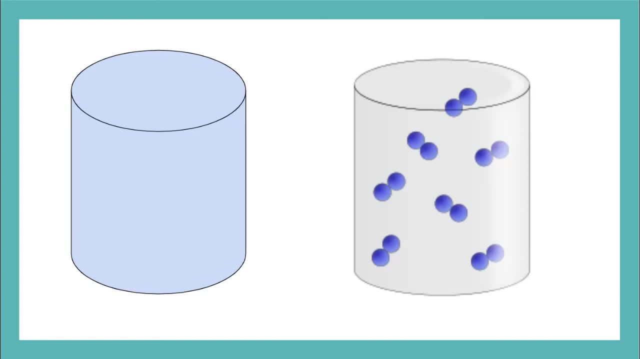 Particles in a gas can vibrate, but they also move at really high speeds. Particles in a gas can vibrate, but they also move at really high speeds. Particles in a gas can vibrate, but they also move at really high speeds. 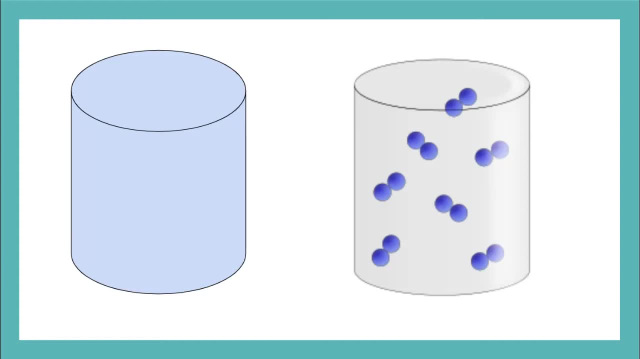 There is a lot of free space between gas particles, and that is why it is easy to compress a gas. There is a lot of free space between gas particles, and that is why it is easy to compress a gas. There is a lot of free space between gas particles, and that is why it is easy to compress a gas. 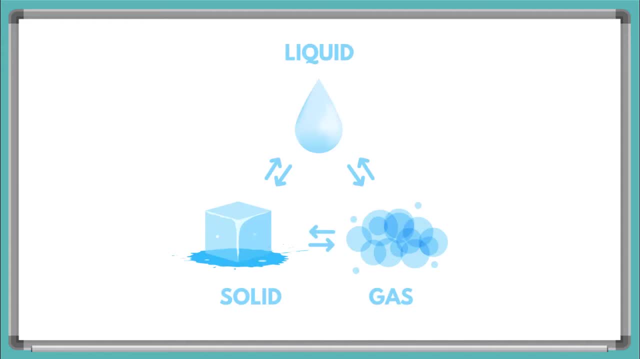 We can change the state. the matter is in. This is called a transition. We can change the state. the matter is in. This is called a transition. Recall that there are four main transitions. Recall that there are four main transitions. Milting, which happens when heat is applied to a solid and it transitions to a liquid. 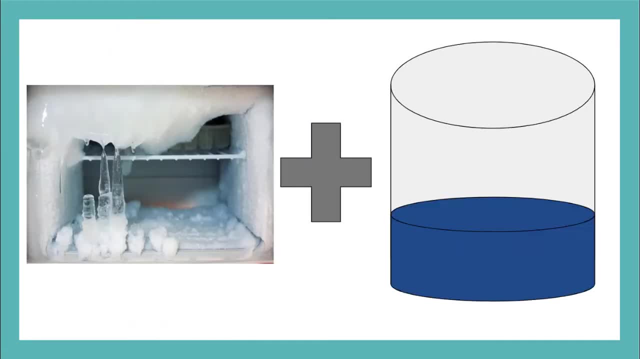 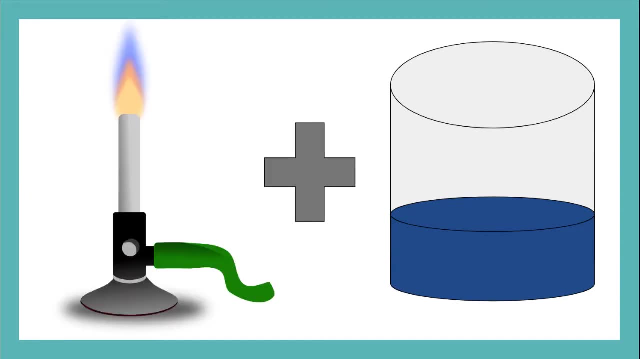 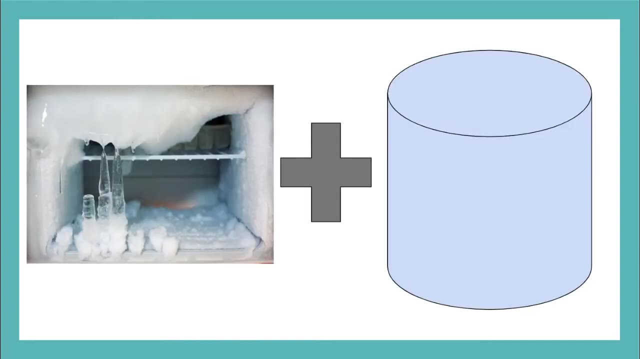 is applied to a solid and it transitions to a liquid. Freezing, which happens when a very cold temperature is applied to a liquid and it transitions to a solid. Evaporation happens when heat is applied to a liquid and it transitions to a gas, And condensation happens when cold. 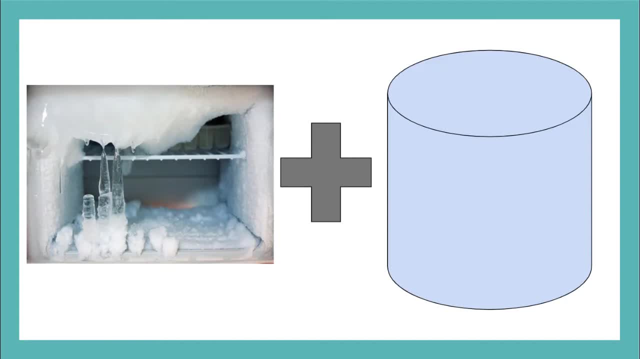 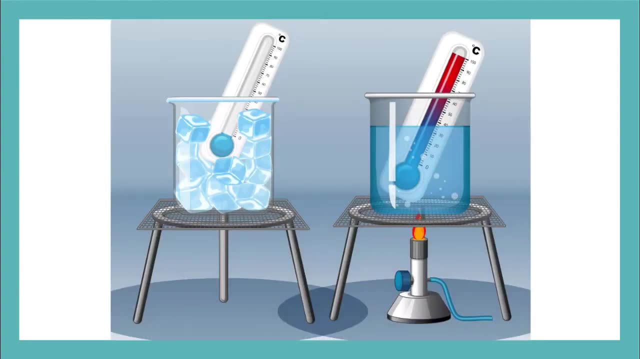 temperatures are applied to a gas and it transitions to a liquid. Do you notice anything about all four of these transitions? Every transition is caused by a change in temperature, And a change in temperature is what we refer to as a change in thermal energy. If you've watched our videos on, 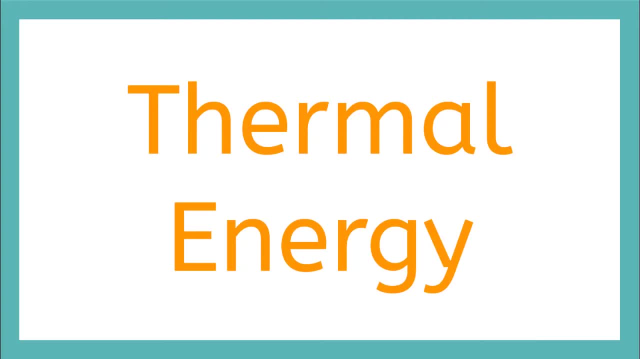 energy. you may know that energy cannot be created or destroyed. So when atoms and molecules have increased thermal energy, they move faster. This is called an energy transfer. But to what kind of energy? To energy transfer. So what kind of energy transfer is energy transfer? It's a. 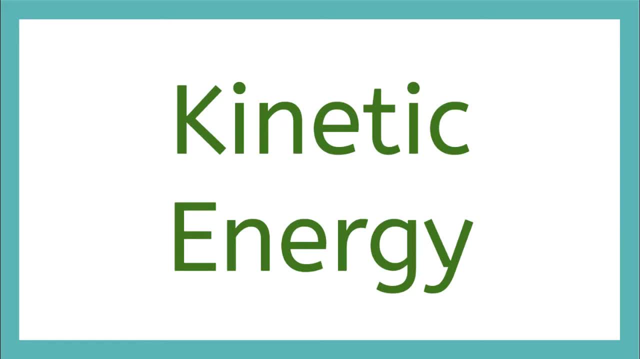 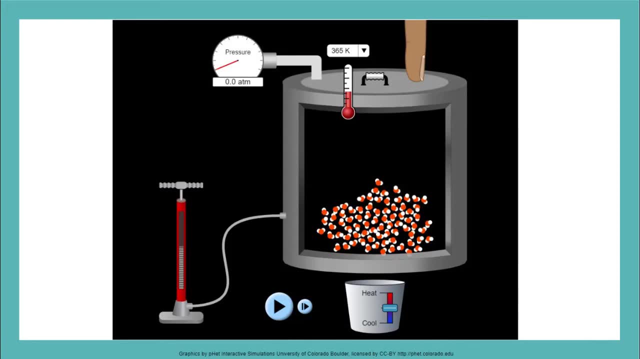 heat transfer. It's not a heat transfer, It's a heat transfer. It's a heat transfer, It's a kinetic energy, the energy of motion. let's head over to a FET game to see what effects thermal and kinetic energy have on the states of matter. so here we are. 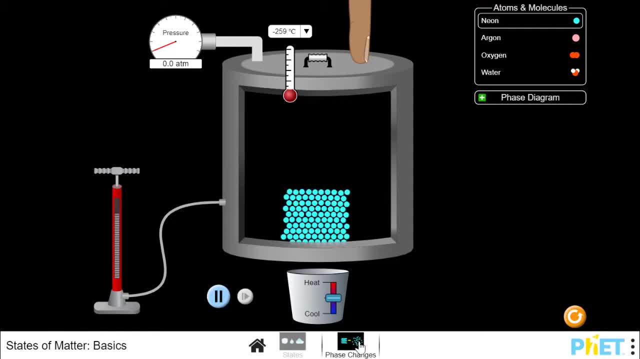 in the FET sim called states of matter, basics, and we're in the second game called phase changes, and you'll see we have four different atoms and molecules that we can choose from. and there's also this handy phase diagram that we will use. I'll show you how to read it. we can change the temperature. here we have a. 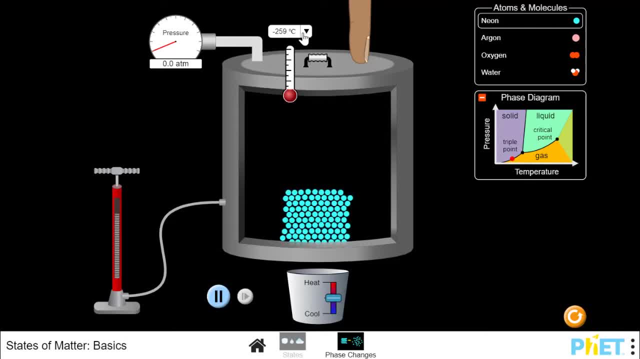 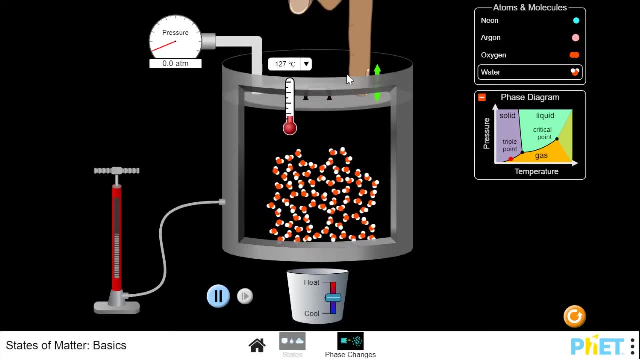 thermometer here. that's either in Celsius or Kelvin. we'll use Celsius because we're going to use water and we will know some of those temperature points. there's also a pressure gauge here, so that's our compressibility. with this finger we can push the lid up or down, and we also have a pump here that. 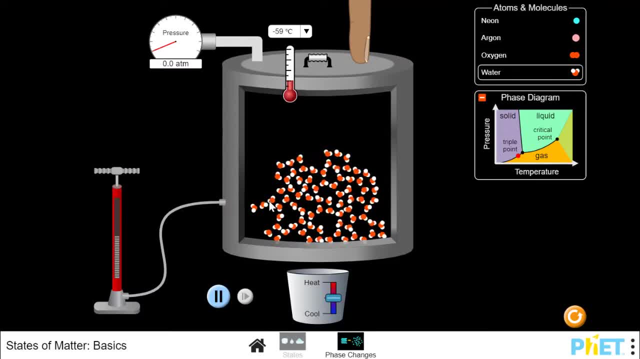 you can add, by lifting it up and bringing it back down, and we can push it up and down, and we can push it up and down, and we can push it up and down- more molecules into your container. all right, so let's get started and see what happens with water. I'm just gonna point out here, with 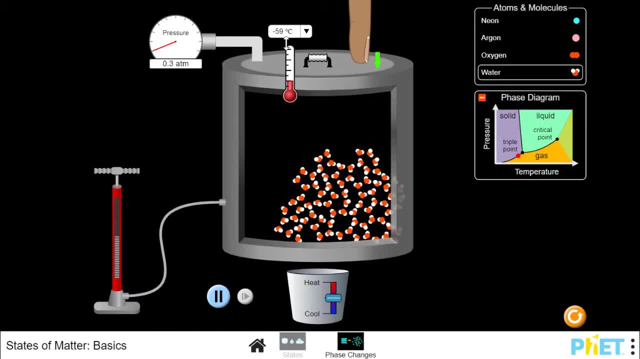 Celsius, the freezing point is zero. so that would mean the water will be a solid and, as you can see here, wherever the red line is, that is what phase we are in. so this black dot will be when our solid turns to a liquid and, up here our liquid, into a gas. 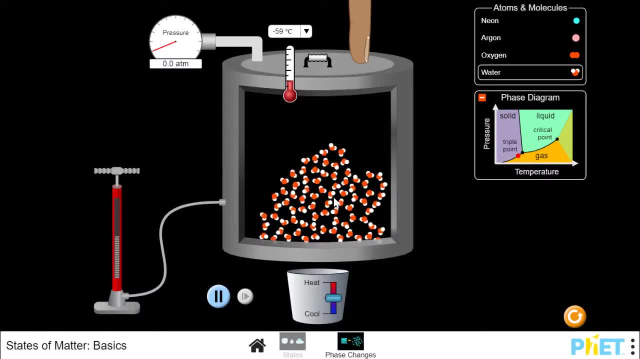 so here we see, our red dot is still on the solid point. so, as you can see, our water molecules are vibrating and jiggling, but me, for the most part, maintaining their shape. so let's increase the temperature here. see, I can lift it up and then bring it back down, and then, if I bring it back to that, zero. 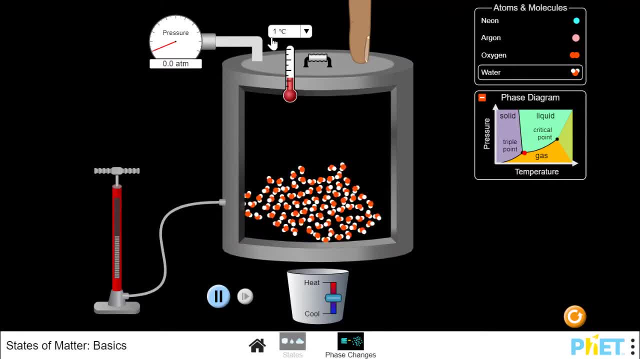 point, it holds it steady. so now I'm at one degree Celsius, at zero degrees is the transition between solid and liquid. you can see now that our molecules are moving on a little bit faster and they're kind of spreading out right. they're taking up the shape here. and what happens now? if I bring the 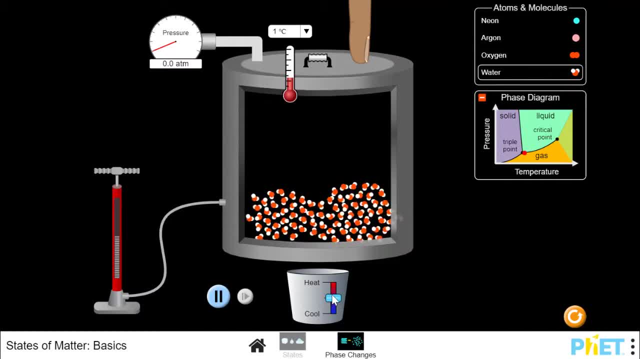 temperature down. look at these molecules, how they're moving. if I bring the lever down, let's say negative 80 degrees Celsius, what happened to the speed that my molecules are moving with it's less now, see, they're just kind of barely vibrating. so let's add some heat again. so I'm going to lift it up a little and that will go. 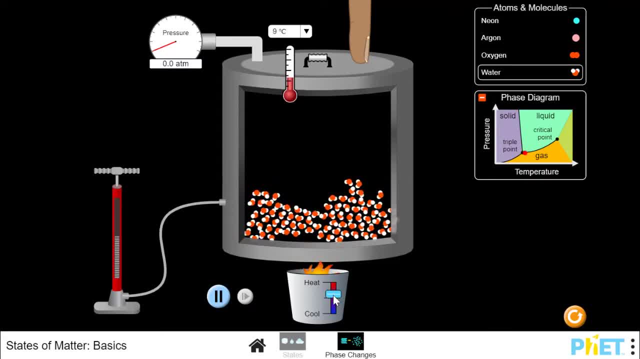 down. see Junع, increasing my thermal energy, I made it 13 degrees Celsius. now you see they're moving a little bit faster. they've spread out into the shape more of how a liquid would look. now let's add some more and see how their kinetic energy so. 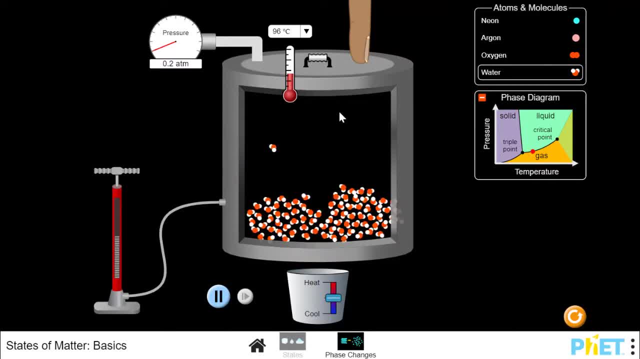 how fast they're moving changes. so now I'm up here at 96 degrees Celsius. so now they're moving pretty fast. you'll see, some of them are even getting an extra boost because they're moving so fast. they're spinning and you see how they have a little bit more freedom they can slide past each other. but right now I'm 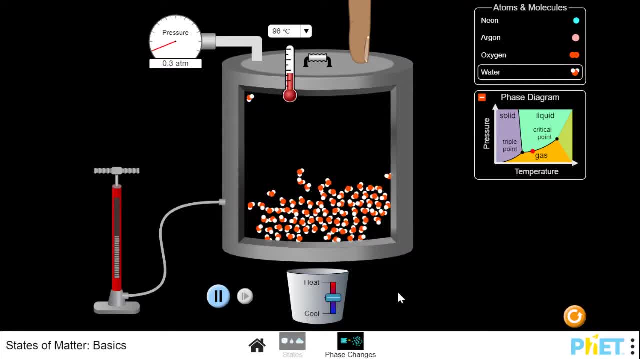 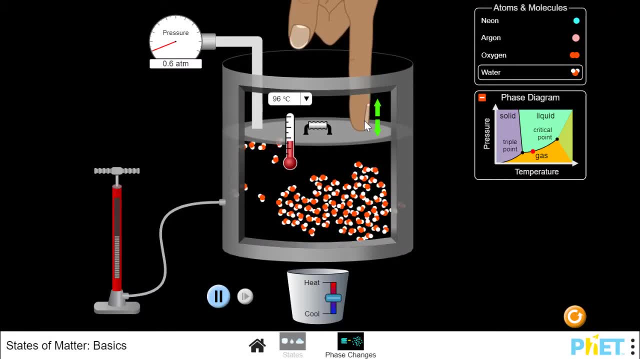 still as a liquid. just some of them are getting an extra boost. let's see what happens as we compress our liquid water. so if I go down to kind of the beginning of where they are, you'll see my pressure is going up. what happened to my temperature? my temperature is going up. 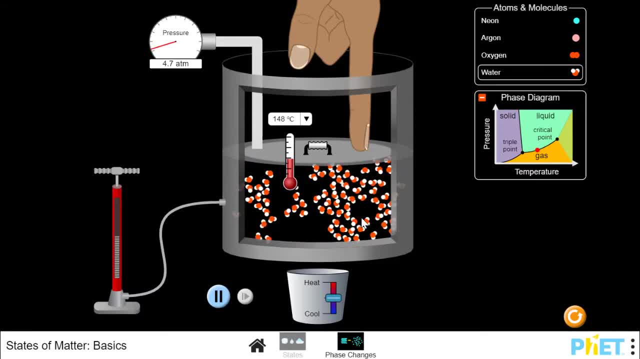 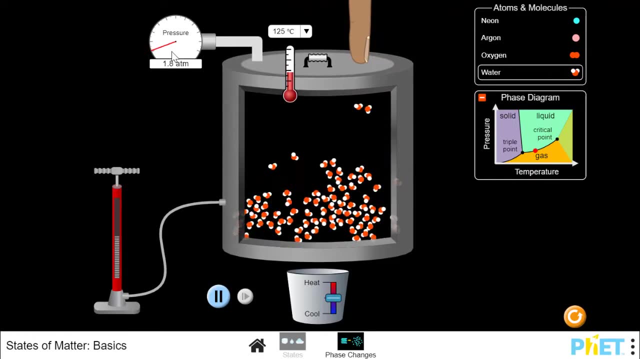 it's also increasing. so that's because, as this pressure goes up, the temperature increases and my little molecules are moving even faster now. so let's relieve our pressure on our liquid water. so I'll see, my pressure gauge is going back down, but these guys are still moving pretty fast. right, my temperature was increased. 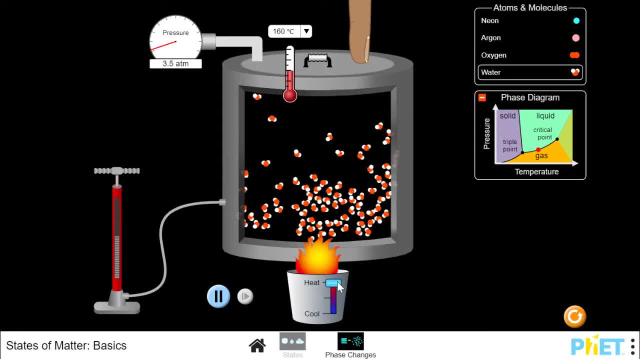 from that let's add some more thermal energy. so I'm turning up the temperature here. you see what's happening to my molecules. are they moving faster or slower? yeah, faster, they're moving crazy and they're taking up a lot more space. and looking over at my phase diagram graph over here, it looks like I'm just. 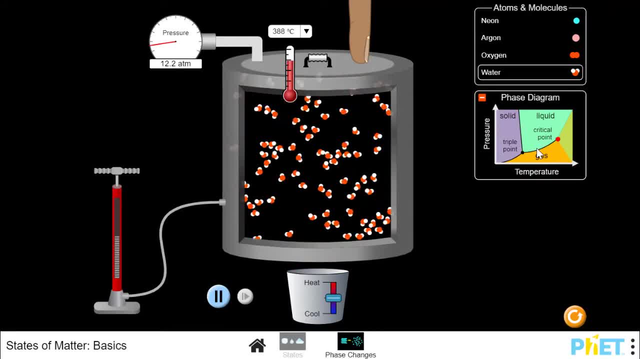 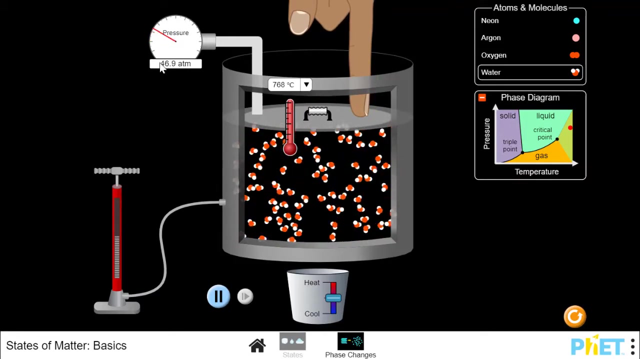 now hitting the gas phase, so I'm right at that transition point and then I'll see these guys. I'm moving freely. there's much more space between them. now what happens if I try to compress my water molecules as a gas? so my temperature increased, my pressure increased, the speed of my molecules increased and take it down a.